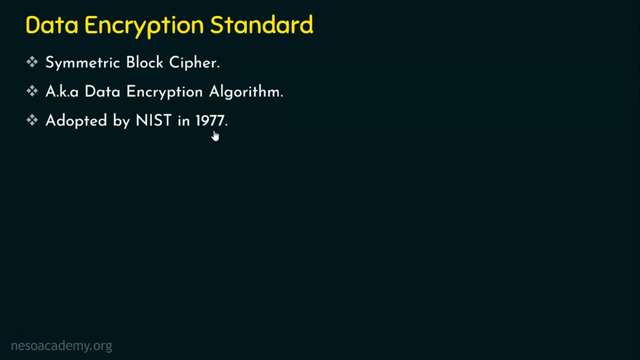 I am not going into the details of the history of the DISS. I am just going to focus on the important perspectives of DISS. DISS is not used nowadays because of the security vulnerabilities And it is completely replaced by AES, the Advanced Encryption Standard, in the year 2001.. 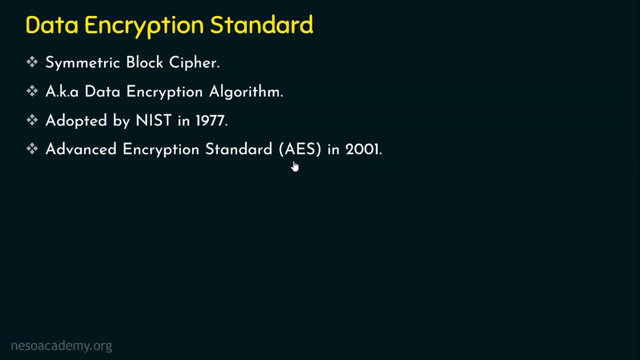 No worries. Anyway, we are going to focus on the AES in this chapter For time being. you just have a note of it that the AES is almost everywhere in today's world. It's so popular because of the powerful encryption algorithm and the encryption standards. 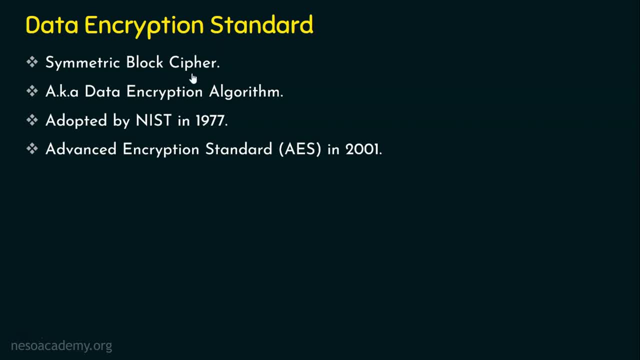 As I already mentioned, this DISS is actually a block cipher, So it's clear that it's not going to take one bit or one byte as an input. Rather, it is going to take a group of bits. Now, how many bits it is going to take? 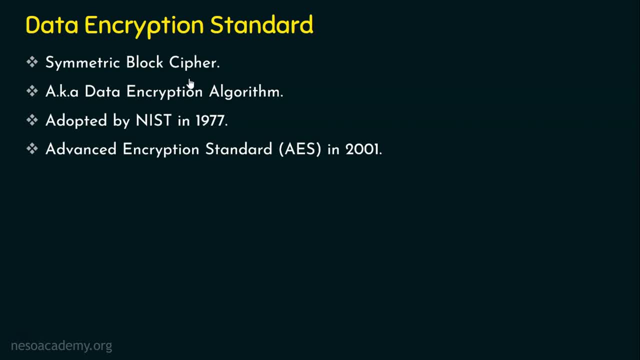 Like: what is the size of the plaintext, What is the size of the ciphertext And what's the size of the key? What is the size of the round key? All this stuff we are going to demystify now. The input size is of 64 bits. 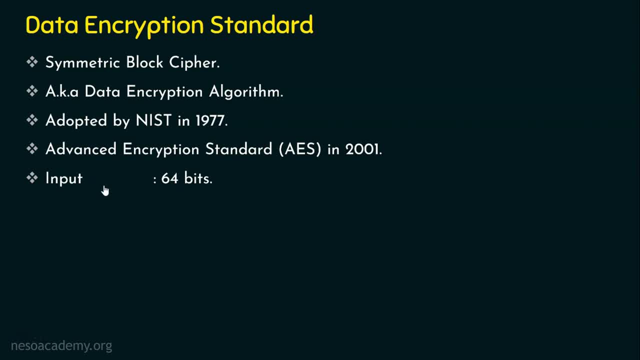 So DISS can encrypt 64 bits at a time. Input means the plaintext, So the plaintext size is 64 bits, And obviously the output size is also 64 bits, So the 64-bit input is fed into the encryption algorithm. 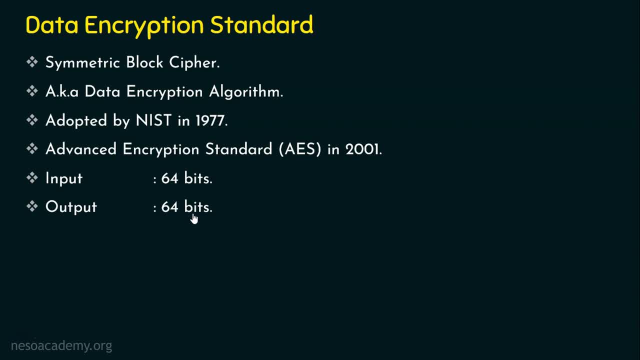 That is the DISS encryption algorithm, And this DISS encryption algorithm is going to convert that 64-bit plaintext into 64-bit ciphertext. Actually, the main key which is given as the input to the algorithm is of 64 bits. 64-bit key is converted into 56 bits. 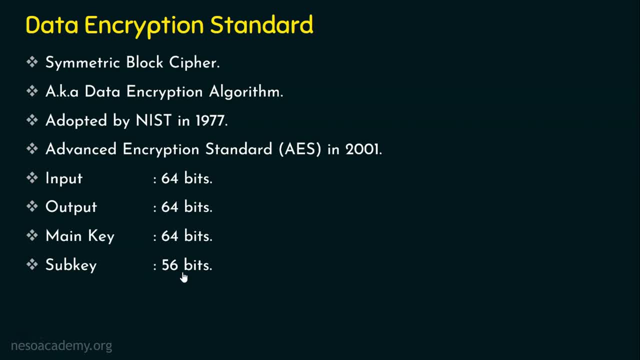 And this is the length of the key we normally refer for DISS. Like we have seen in the Feistel structure, we have n number of rounds Here also, we are going to have some fixed number of rounds. Let me tell you how many rounds are there shortly. 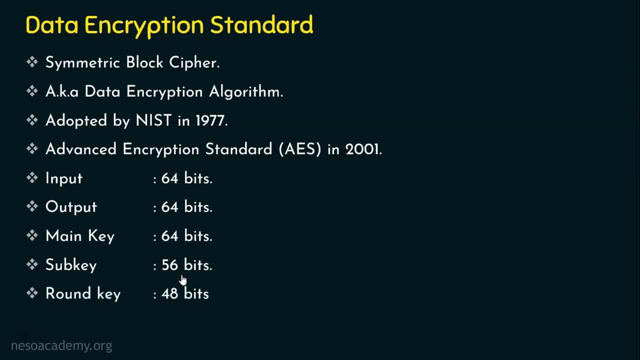 But for all these rounds we need round key, And the size of the round key is 48 bits. Then how many rounds are there actually in DISS? There are 16 rounds in DISS, So for 16 rounds we need 16 round keys. 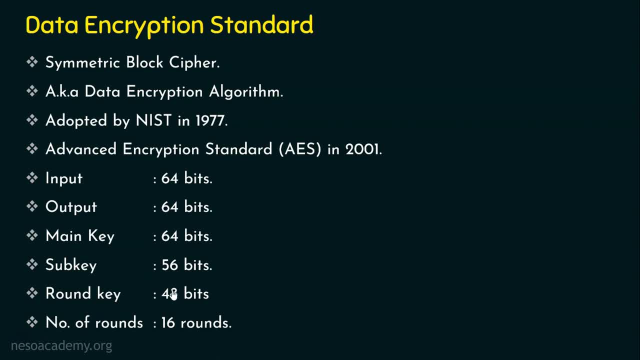 And how these round keys are generated. These round keys are generated using this 56-bit key length. Actually, this 56-bit key is helping the DISS algorithm to generate 48-bit round keys. How many round keys? 16 48-bit round keys. 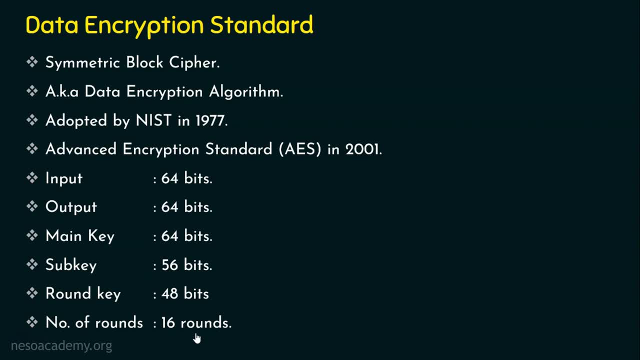 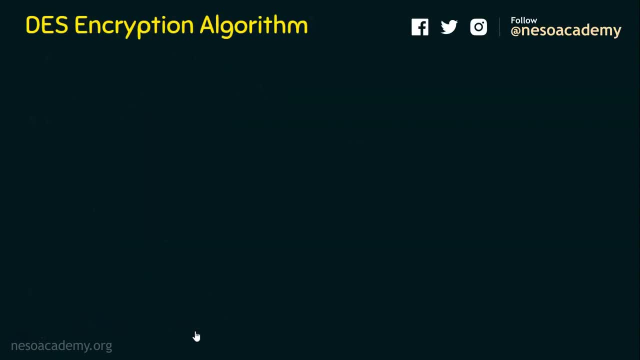 So this is the actual basics that are required for understanding the DISS. Let's dive into the encryption algorithm. So we are sure that DISS is a block cipher, and what's the size of the input and output, The plaintext and the ciphertext, I mean? 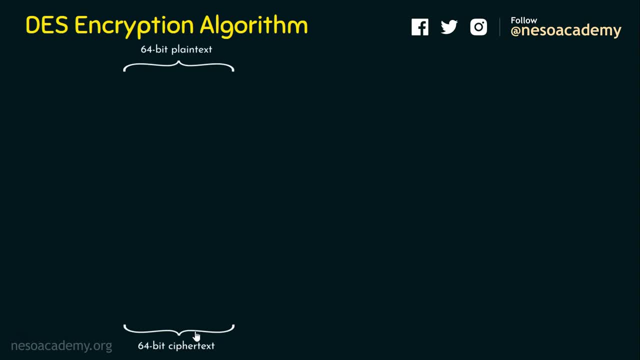 So the input is 64-bit and the output is also 64-bit. So DISS is going to take a 64-bit plaintext and it's going to convert this 64-bit plaintext into 64-bit ciphertext, And that is why this is actually called as a block cipher, because it is taking a group of bits. 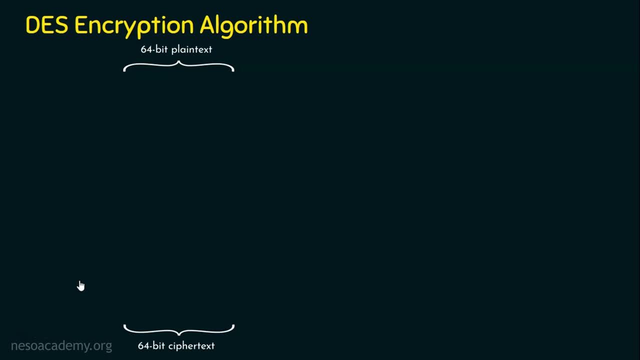 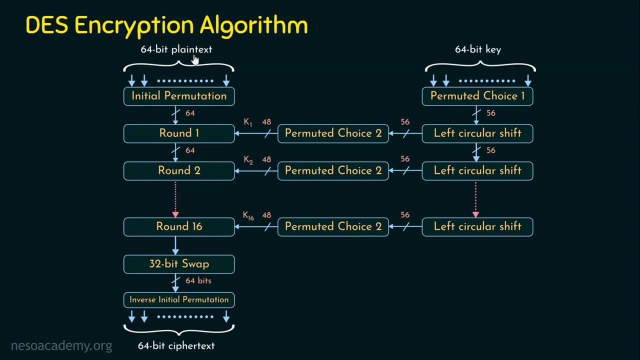 What is happening inside this encryption algorithm. Let me unbox this. So here is the DISS encryption algorithm. If you see, here the 64-bit plaintext is actually going to be converted into 64-bit ciphertext, And this 64-bit plaintext is actually. 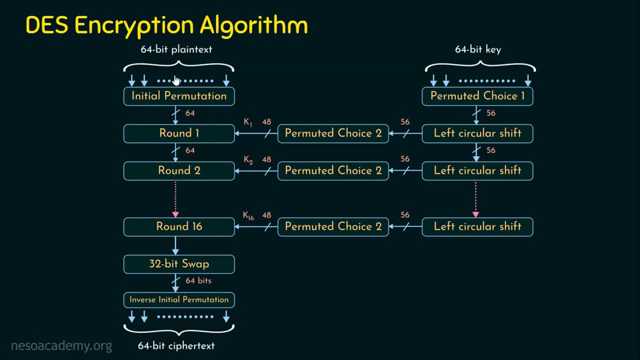 given to this initial permutation function. So 64 bits are sent to this function And after doing a permutation it gives 64 bits as the output. So it's clear that the 64-bit plaintext is given to the initial permutation function and it gives 64 bits. 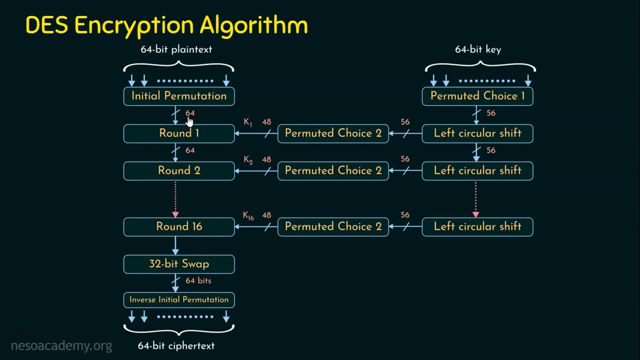 Now, how many rounds are there? As I mentioned earlier, there are 16 rounds in DISS. So here is round 1, round 2, up to round 16.. Now, if you see here for every round, 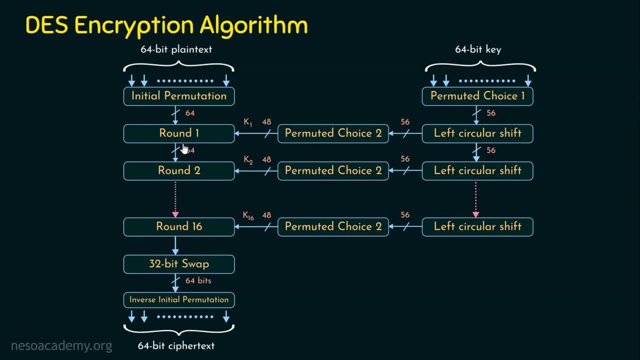 64 bits are given as the input and the output of every round is going to be another 64 bits, And what is happening in this round That I am not going to touch upon in this presentation. We will focus on that in the next presentation. 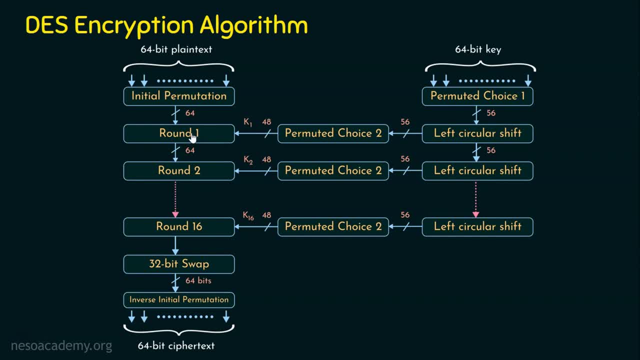 So for now, just understand: 64 bits input is given to each round and the output of each round is going to be 64 bits. So, likewise, we are processing 16 rounds At the end of 16 rounds. whatever we get, is this the ciphertext? 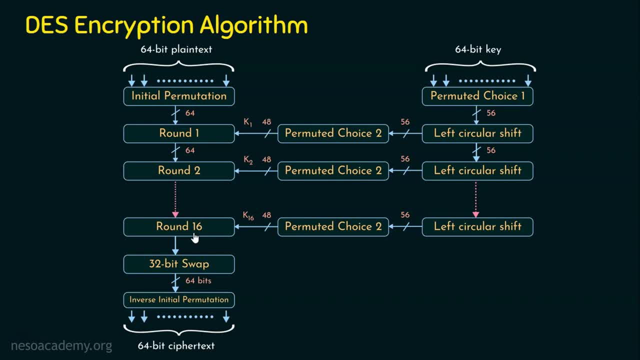 No, This is in the Feistel structure what we have seen. After completing the n rounds, whatever we get is the pre-output, So it needs to be swapped right. So after 16 rounds of operation, we get 64 bits, and these 64 bits are given to a 32-bit swap function. 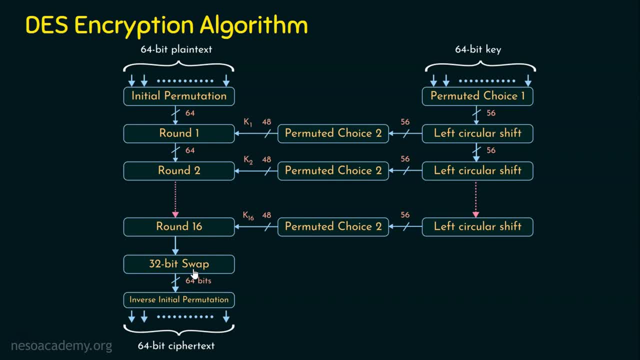 So if you take the 64 bits, we can partition this into left-hand side 32 bits and the right-hand side 32 bits. Just perform a swap. Once the 32 bits are swapped again, we'll be getting 64 bits only because 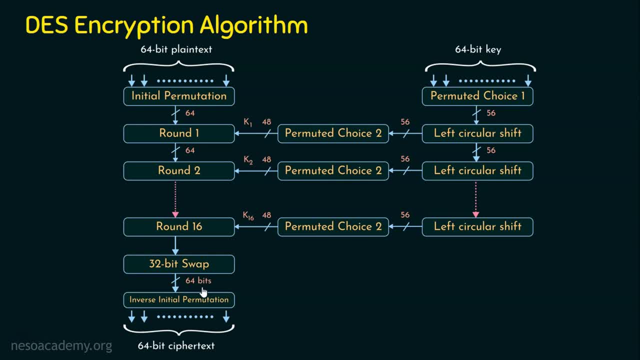 the left-hand side, 32 bits are going to be placed in the right-hand side and the right-hand side 32 bits are going to be placed in the left-hand side. So it's clear that the output of the 32-bit swap function is going to be 64 bits. 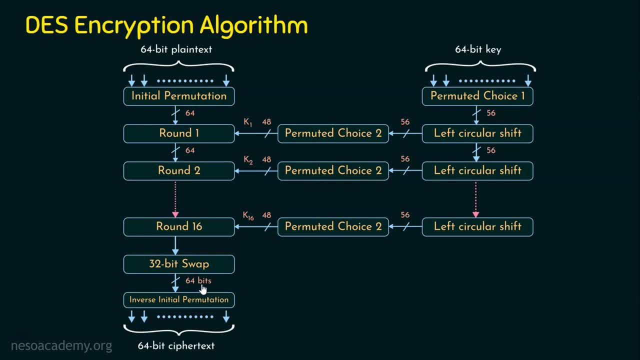 Now, this is also not the ciphertext. Just recollect what we did in the starting part of the encryption process. The 64-bit plaintext is actually fed into the initial permutation, right? So we need to inverse it. So the output of this 32-bit swap function is going to be 64 bits. 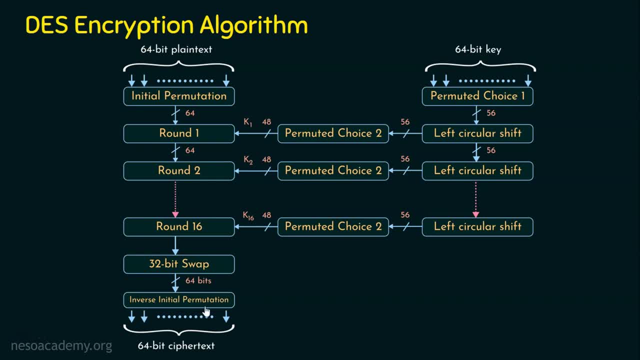 and these 64 bits are given to the inverse initial permutation function, which inverses and then gives 64 bits, and these 64 bits are the ciphertext bits. So it's clear that the 64-bit plaintext is converted into 64-bit ciphertext. 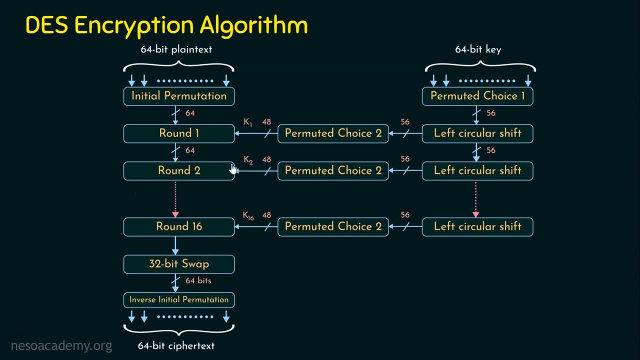 And, if you see, here there are 16 rounds And, as I already mentioned, for each round we need round keys and the size of the round key is 48 bits. So K1 is the round key for round 1, which is 48 bits. 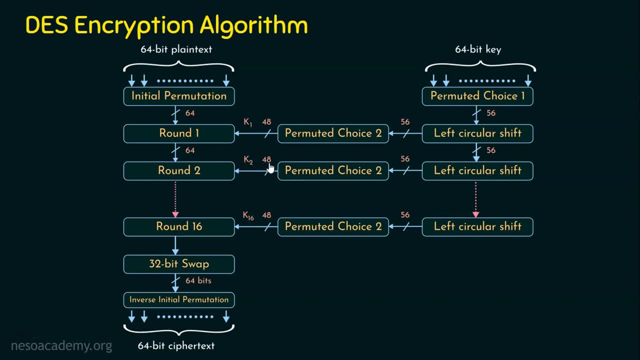 Similarly, K2 is the round key for round 2, which is also of 48 bits. Likewise, we have 16 round keys and K16 is the round key for round 16, which is also of 48 bits. As I already mentioned in the previous slide, the size of round key is of 48 bits. 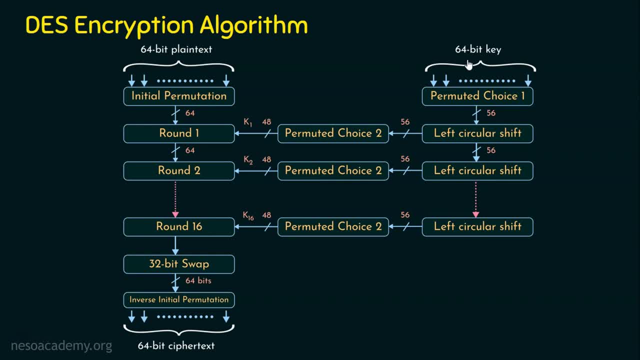 But actually this encryption algorithm starts with the 64-bit key, But this 64-bit key is actually converted into 56 bits And this 56-bit key only is actually used for generating the round keys, which is of 48 bits in nature. 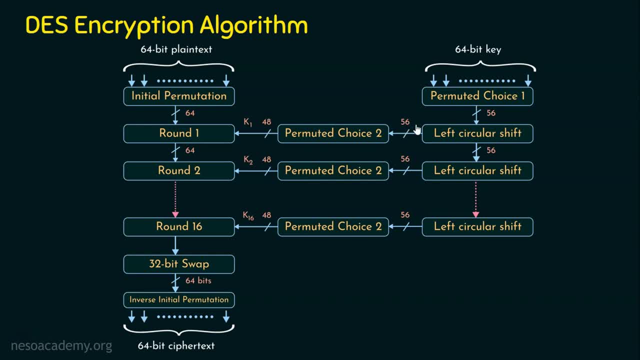 So the key length is 56 bits in the DES algorithm. Before we conclude, let's see what are all the things that we are going to see in the next presentation. We are going to focus on the first one, the initial permutation. 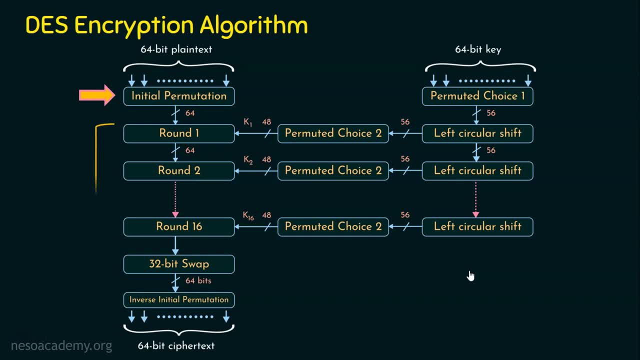 So we will be understanding what happens in the initial permutation, Then we'll be focusing on the round function and then we'll be focusing on inverse initial permutation And later we will see what happens in every round. And that's it, guys. 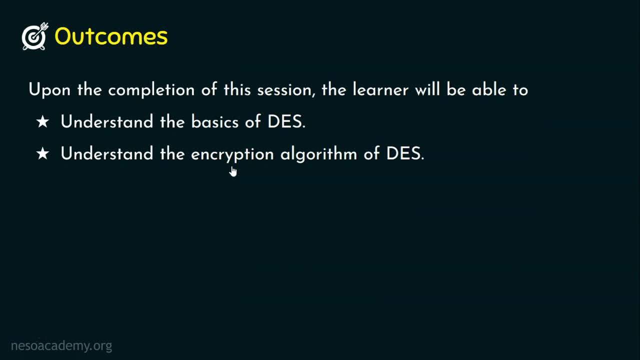 I hope now you understood the basics of DES and we also have understood the encryption algorithm of DES. I'll see you in the next presentation And thank you for watching.